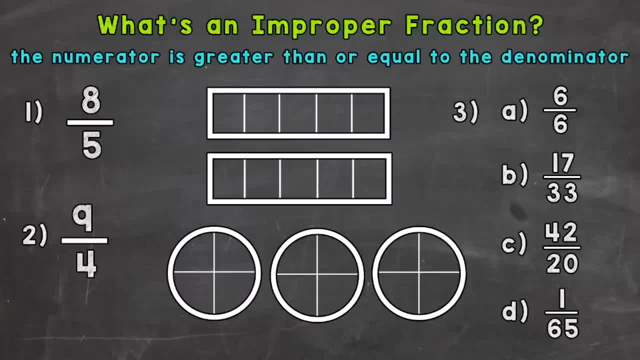 Let's take a look at modeling this fraction to show how it is greater than one whole, So 8 fifths. I have two whole rectangles to the right here, So we need to fill in 8 fifths. Each rectangle is cut into fifths, so we need to fill in. 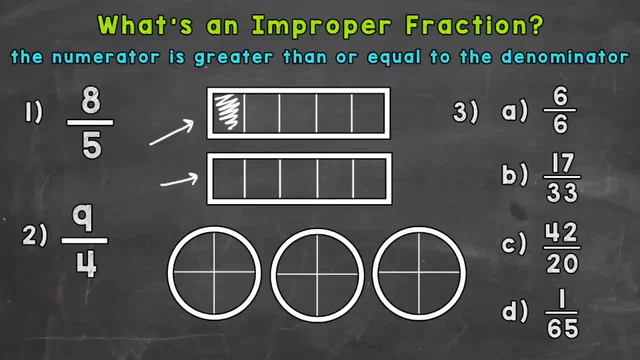 8. So, for example, this would be 1 fifth And we have 2,, 3,, 4, and 5.. So right now we're at 5 fifths, 5 out of 5 filled in, And I want to mention whenever we have the same number. 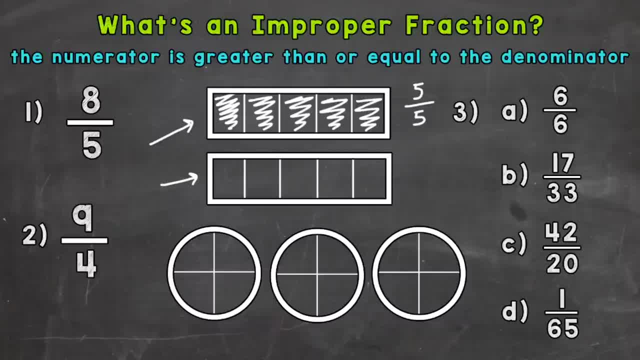 up top as we do the bottom. when it comes to fractions, we have an improper fraction and that fraction equals one whole. So whenever you have the same number on the top and bottom, it equals one whole. But we need to continue here for number one, because we need to get to 8.. 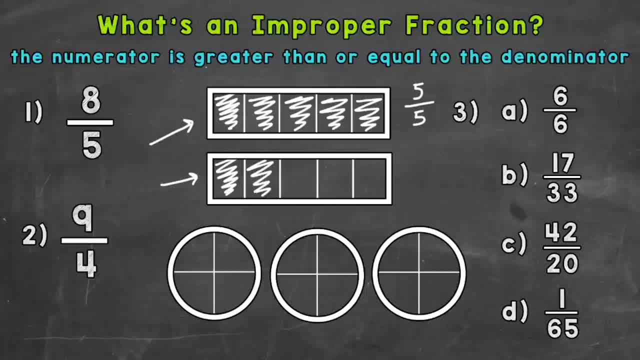 So this would be 6,, 7, and 8 fifths. So you can see that we have one whole rectangle filled in and then 1,, 2,, 3 fifths. So 8 fifths equals 1 and 3 fifths. 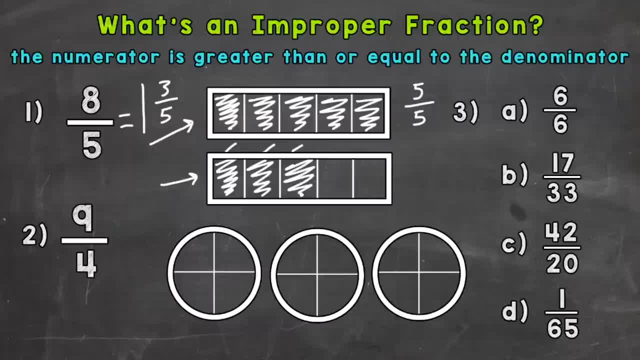 And we can see that that has a value greater than one whole. It's an improper fraction. So let's take a look at another example. For number two. we have 9 fourths. So 9 fourths- the numerator- the top number- is greater than the denominator, the bottom number. So we have 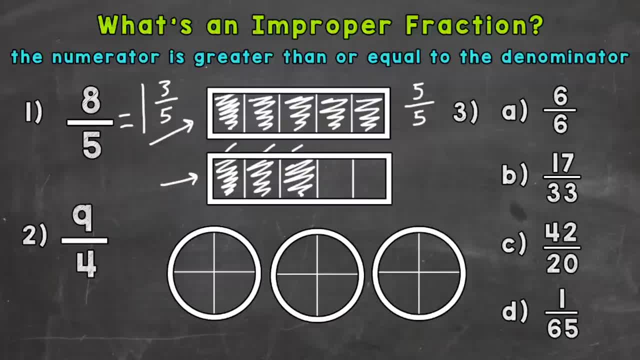 an improper fraction, And this improper fraction's value is going to be greater than one whole. If we were to have- I want to mention this again because it's important- if we were to have 4 over 4, remember same number up, top and below. 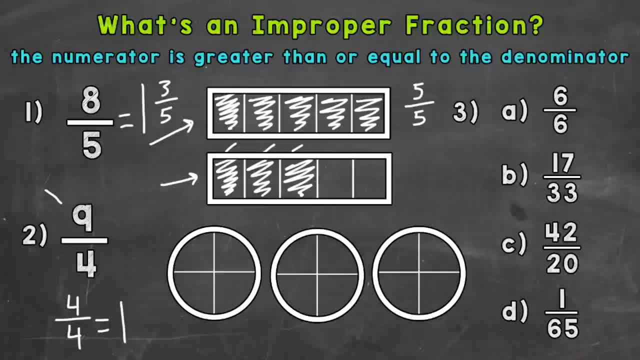 equals 1.. But in the case of number two, 9, fourths. that top number is greater than the bottom. So this is going to be greater than a whole, And let's model this one. So we have holes to the right here, whole circles, and they are each cut into fourths. 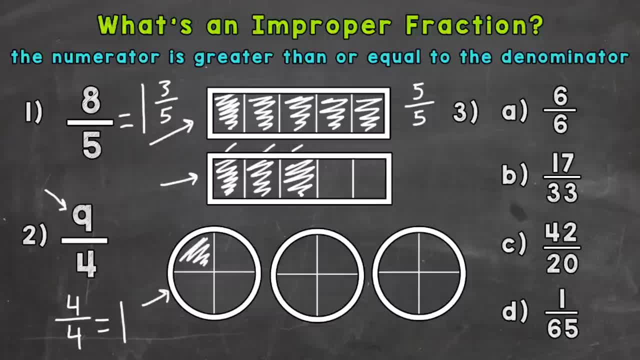 So we need to fill in 9 fourths. So 1,, 2,, 3, and 4 fourths, So you can see one whole there: 5,, 6,, 7,, 8, and 9.. So we have two whole circles filled in, and then right here we have one fourth. 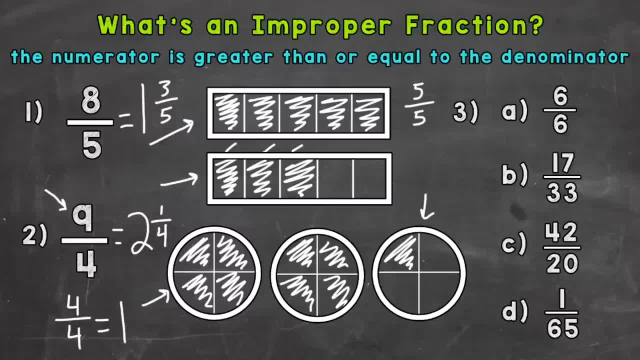 So 9 fourths equals 2 and 1 fourth. So I want to mention that this is an improper fraction. Now, right over here, where we have a whole number and a fraction, that's called a mixed number, And improper fractions and mixed numbers are equivalent. 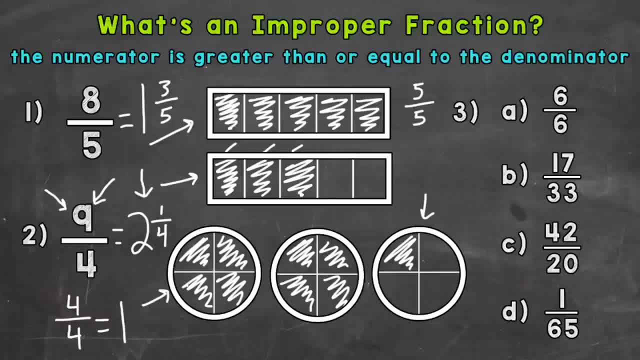 just in complete fractional form. and then the other shows the whole number plus the fractional form. But nine-fourths and two and a fourth are equivalent, Just like number one. eight-fifths and one and three-fifths are equivalent. So as far as number two, I'll wrap this one up by saying that: 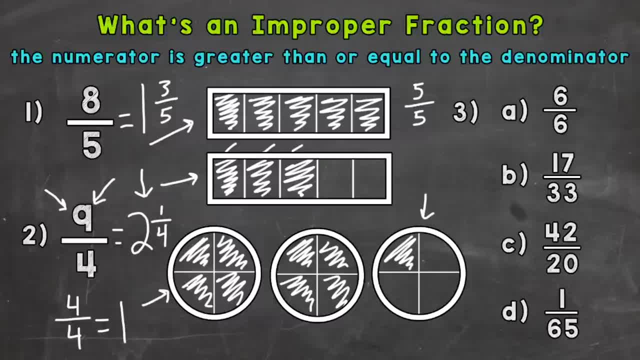 we proved that nine-fourths is greater than a whole. there, And again we had an improper fraction because the numerator was greater than the denominator. So let's move on to number three, where we have four choices- a, b, c and d- and we need to pick out which ones are improper. So let's 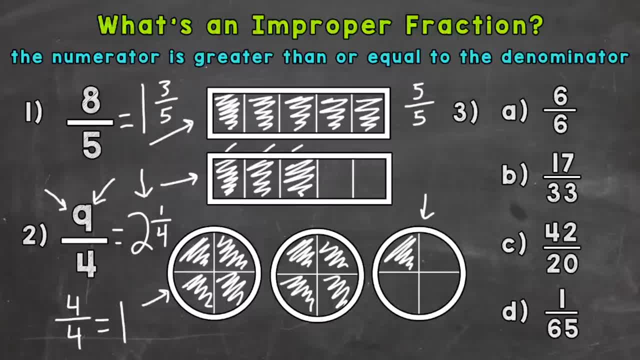 start with a, where we have six-sixths. So our numerator, the top number, is the exact same as the denominator. Therefore this fraction equals one whole And in the case of this our numerator is equal to the denominator. So we have an improper fraction. Choice b: we have 17 over 33.. 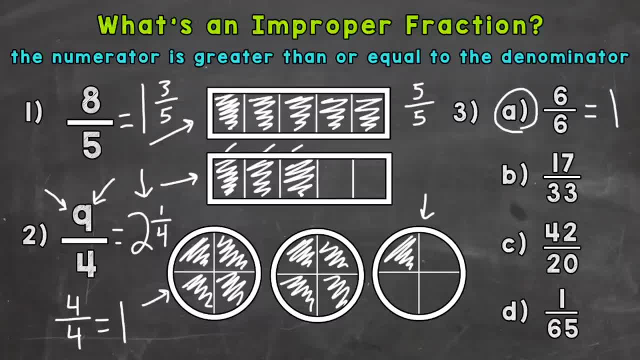 So the numerator is less than the denominator. That's what we call a proper fraction. So this is not improper. Now choice c: our numerator 42, is greater than our denominator of 20. So we have an improper fraction there. And lastly d, we have one over 65.. So the numerator is less than the denominator. Choice d: 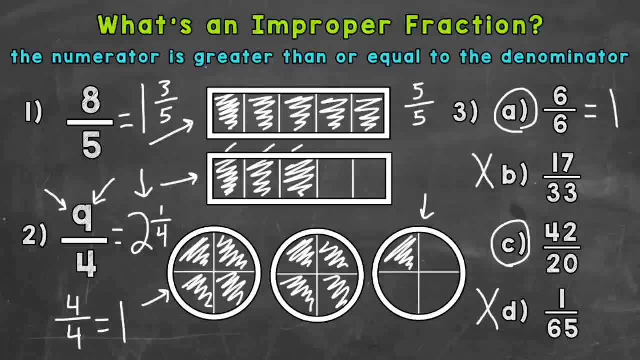 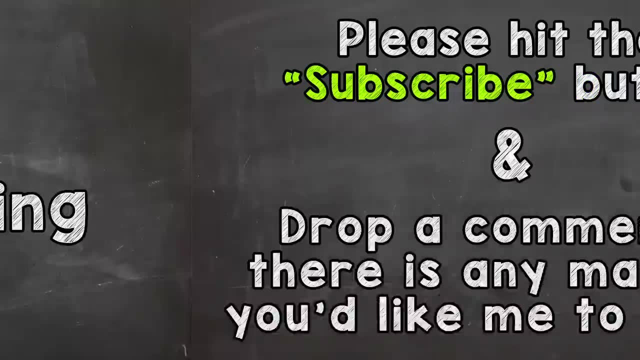 is proper, Therefore not improper. So there you have it. There is a brief introduction into improper fractions and some examples to show exactly what they look like and what they are. So I hope that helped. Thanks so much for watching. Until next. time peace.